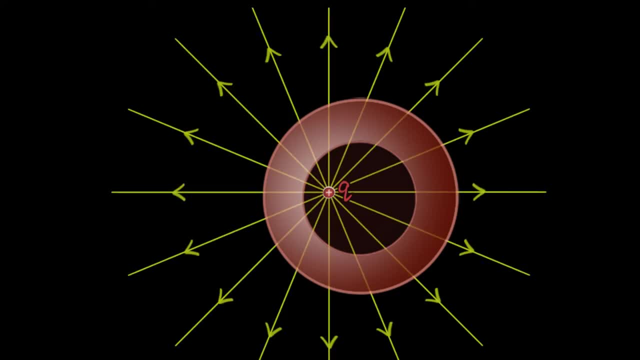 See, this positive charge is gonna start producing an electric field And that electric field is gonna start sucking the electrons from this metal. Remember, metals have free electrons. They can move under the influence of electric field. So as a result of that, electrons will get sucked in. 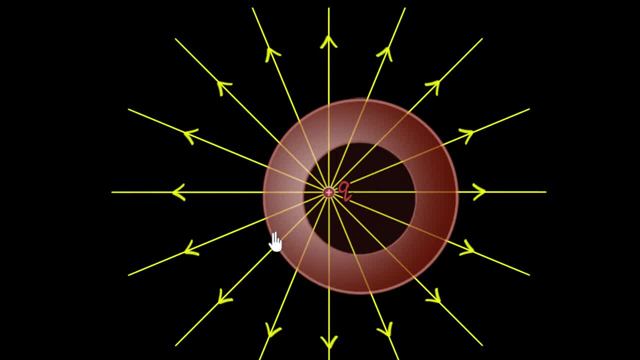 And so there will be some negative charge getting induced over here. As a result of that, there will be some positive charge getting induced on the outer surface And, as a result of that, our electric field is gonna get modified. So the question is: once all the electrons 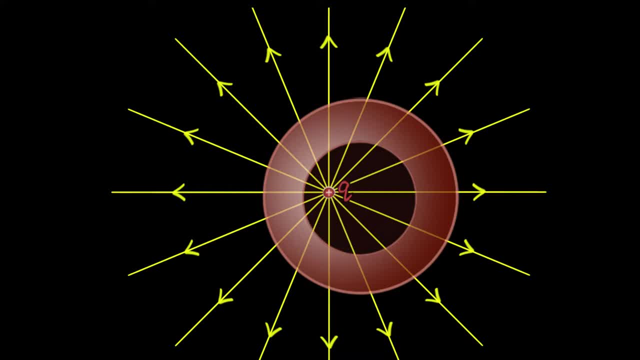 have stopped moving. once we have reached electrostatic condition, we have to answer three questions. What will be the total charge on the inner surface and how the distribution would be? What will be the charge on the outer surface and how the distribution would be? 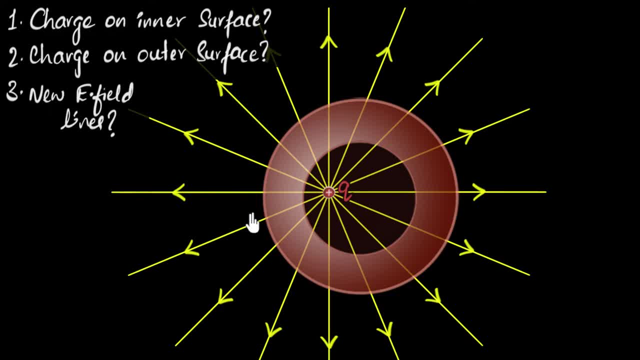 And what would the new electric field lines- roughly the sketch of that- how would that look like? So these are the three questions we're gonna try and answer. So how do we do this? Where do we even begin? This looks like a very complicated, challenging puzzle. 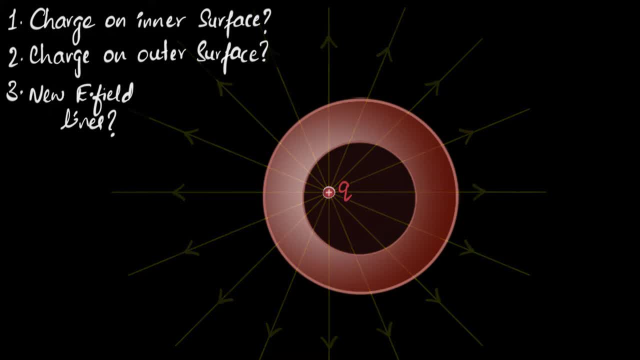 But what I like to do, let me first dim the electric field lines a little bit, All right, So what I like to do is go back to one of the basic things we've seen about conductors and electrostatics. You've seen that in electrostatic conditions, 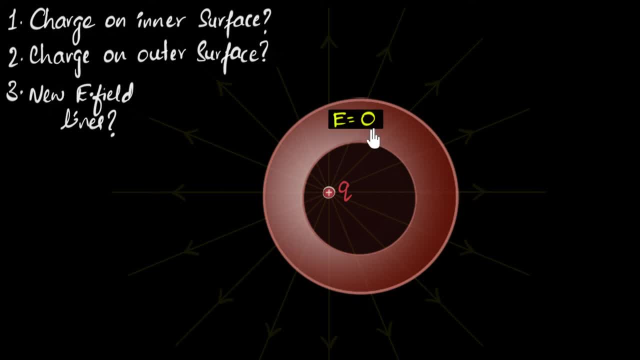 conductors should always have zero electric field inside of them. Why? Because if there are any electric fields over here, they will start pushing on this electric field and the electrons will start moving. that means we are not in electrostatic condition, because electrons are moving. 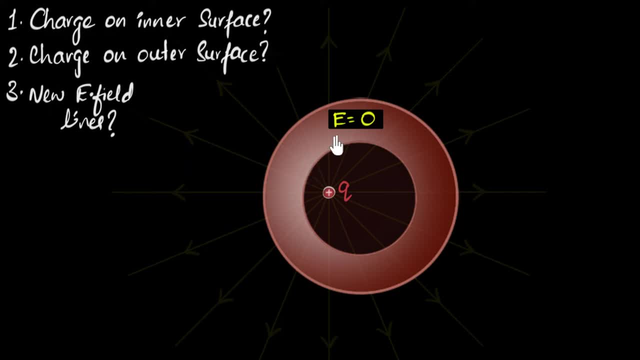 So whenever we are in electrostatic condition, automatically, it means that there are no electrons moving. automatically it means that the electric field must be zero. And if you need a more refresher on you know on this concept, we've talked about this in great detail. 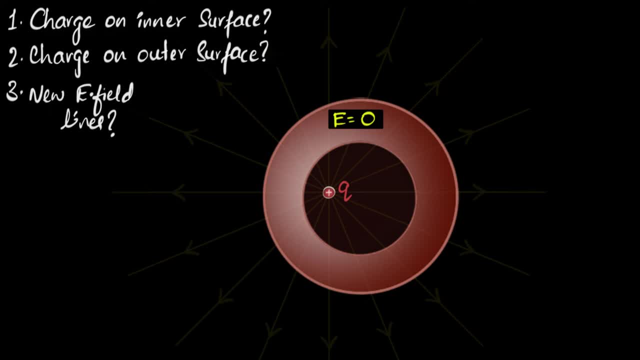 in a previous video on electrostatic shielding, So feel free to go back and check that out. But anyways, let's come back to our question. We know because of this, of this electric field generated by the positive charge, it's going to start, you know, sucking in. 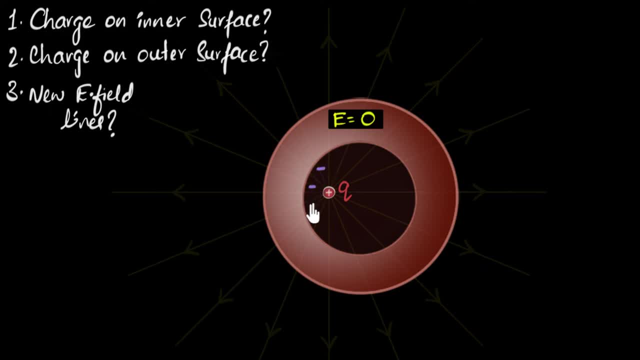 negative charges. so there will be some negative charges over here. and because our conductor is neutral, if there are some negative charges which are induced over here because of that, some equal number of positive charges should get induced on the outer surface. so there should be some positive charges induced on the outer surface and our goal is to figure. 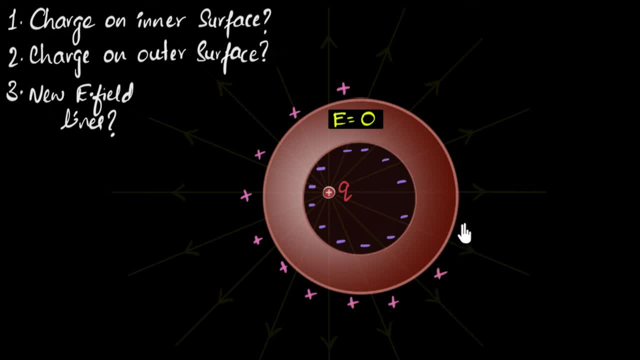 out how much these are okay, because we are given that this in inner charges plus q. so let's start with the induced inner charges, the purple charges, negative charges: how much would that be? would it be equal to negative q? would it be more than negative q? would it be less than negative q, or do you think it's possible? do you think it? you know there is. 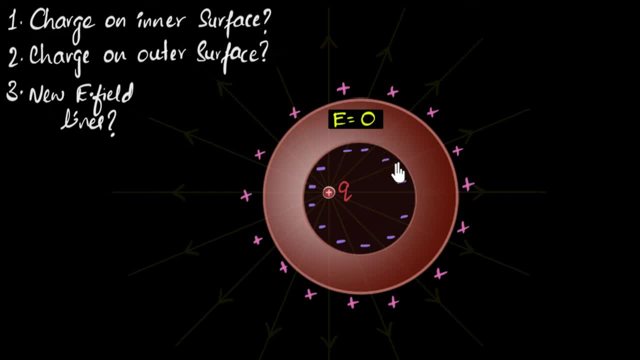 no info, not enough information, we'll not be able to calculate that. how do we do this? how do we figure out how much these are? okay, because we are given that this inner charges plus q could be well. at first it looks like how do i know? like how would i know in the electrostatic situation? 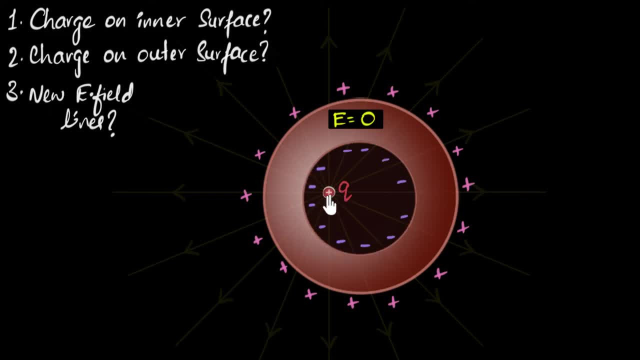 exactly how much of the negative charges would come. maybe it depends upon the position of this charge, maybe it depends on the strength of this charge, i don't know for sure. so how can i calculate that? well, we can use this to our advantage. we know that the electric field has to be zero, so the 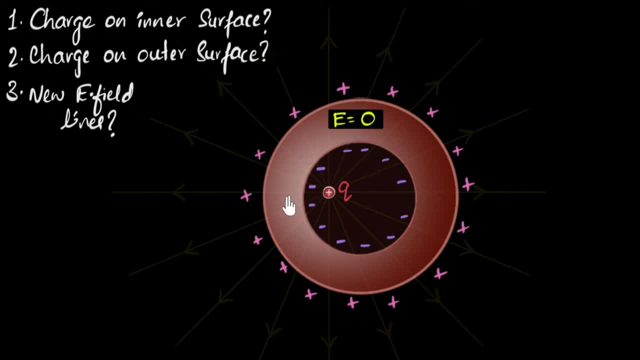 negative charges induced must be in such a way that they should kill the electric field over here. but how? how do i figure out exactly how much? what is the connection between charges and electric field? oh, gauss's law. gauss's law is the one that connects charges and electric field. so why don't you pause? 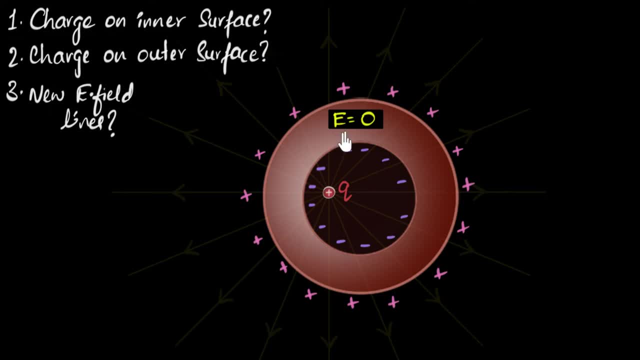 the video and see if you can somehow use gauss's law to figure out exactly how much negative charge should be induced inside. so why don't you pause the video and think about that? so what i would like to do is i'm going to choose a gaussian surface and make sure that gaussian surface 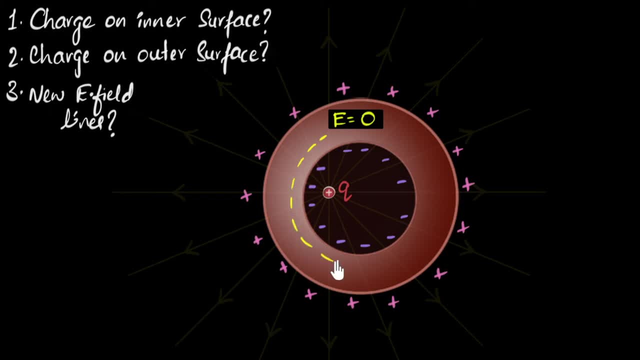 the entire surface. choose a sphere, and i'm going to choose a gaussian surface and i'm going to choose a sphere, but the entire surface lies within the bulk of the conductor. so imagine, this is my spherical gaussian surface. now, because i know that under electrostatic conditions, electric field 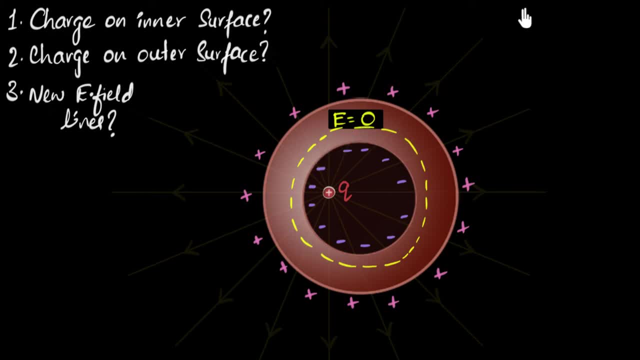 everywhere over here is zero. therefore i know that the total flux through that surface must be zero. so net electric flux must be zero, which means that the total enclosed charge must be zero. and from that i think i now understand how much this negative charge should be. if the total enclosed charge should be zero- and i already have plus q- that means the total negative. 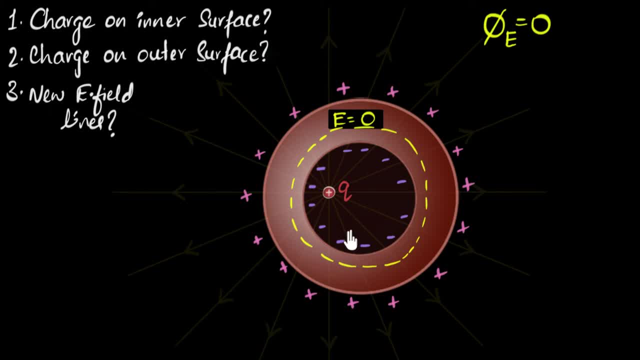 charge must be negative q. so this should be negative q. only then the total enclosed charge becomes zero. and what's amazing is that it doesn't matter where i position this, this little q, it doesn't matter where i move it. the total induced must be negative q and therefore the total induced on the outer surface should be. 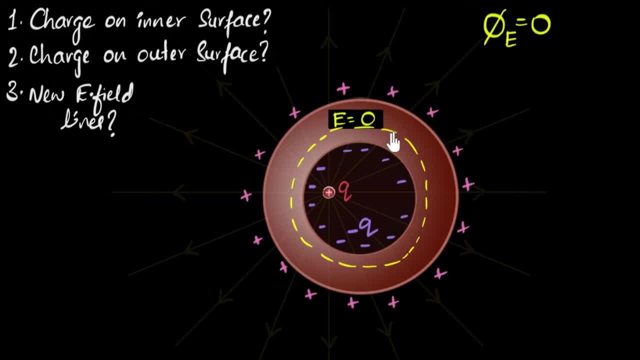 plus q. it has to be because we know that the conductor is neutral. so if there is negative q inner induced on the inner surface, plus q must in get induced on the outer surface. so the charge on the outer surface is plus q, the charge on the inner surface is negative q. and so what's interesting? 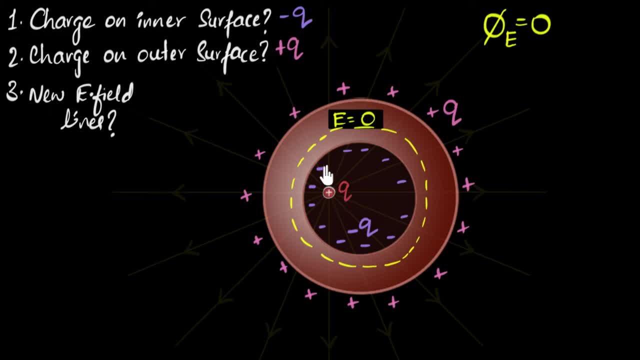 is, whatever charge we introduce inside, automatically that charge gets manifested on the outside. wonderful, isn't it? that's an amazing thing about a conductor. but we're not done yet. we also need to look at the charge distribution and what the electric field looks like, what the new electric field is going to look like. so let me bring back the original electric 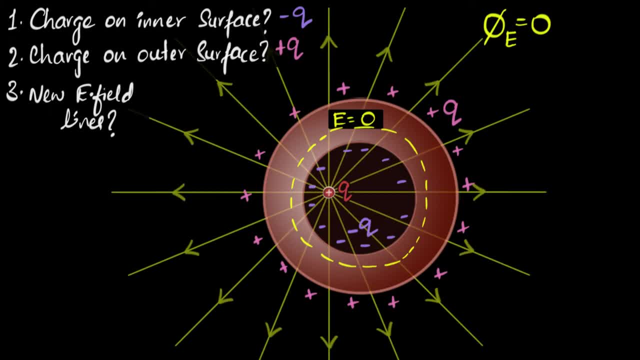 field. here it is. so this is, this would have been the electric field at the beginning, before all of these charges got induced. the question is, what would this new electric field look like? let's do this in steps. let's first look at the electric field in this region. what's going to happen to that? we know. 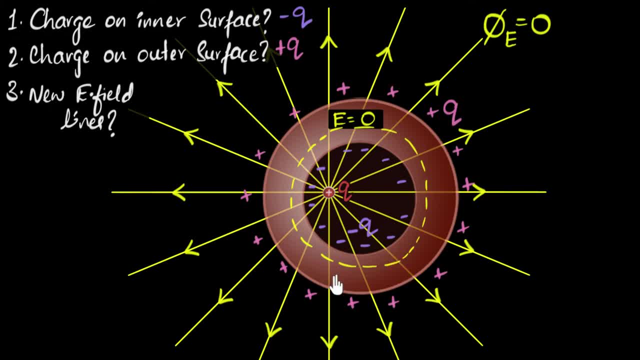 that electric field has to be zero in understanding electrostatic conditions, so we can go ahead and drop that. so let me do this. this electric field is going to disappear, all right, so we got one part solved. the next question i want to try and answer is: how would the new electric field inside? 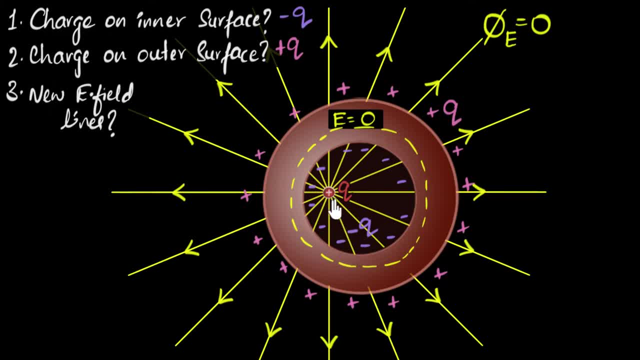 look like? would it look exactly this way, which would just look like this, or do you think it's going to change again? can you pause the video and think a little bit about this? all right, we know that, because the entire conductor has zero electric field. it's an equipotential surface, again something that we have. 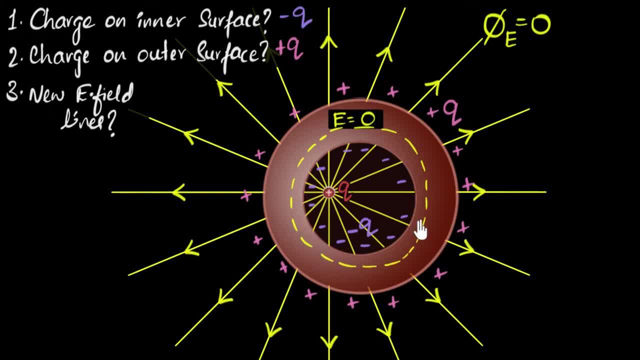 talked about in previous videos. but because our conductor is an equipotential surface, that means the electric field over here must always be perpendicular to the surface, and you can see that these electric field lines are not over here. they're not perpendicular, which means these electric field lines are going to bend in such a way that they try to be perpendicular to the surface. 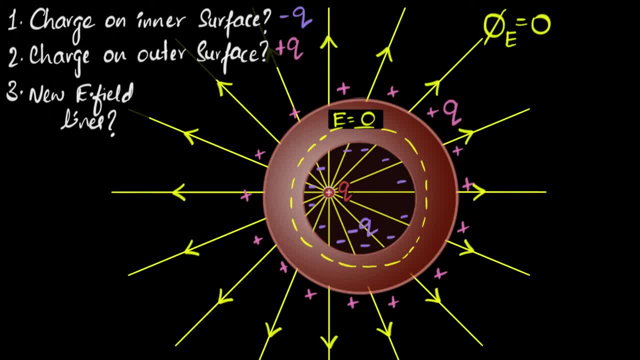 so the way it's going to look like again, it's a rough, rough figure. the electric field lines are going to bend somewhat, like this, from positive to negative, but they also always ensure that the angle between the field lines and the inner surface is going to be 90 degrees. all right, i. 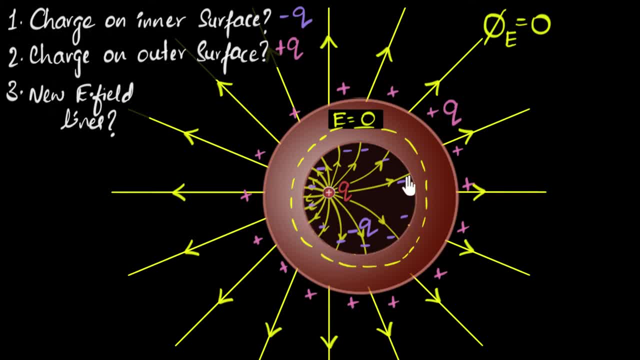 have another question for you. how do you think would the charges get reduced? uh, this, how would the charges charge distribution look like? do you think it's going to be a uniform charge distribution over here, or do you think there's going to be? you know, some, some part is going to have more. 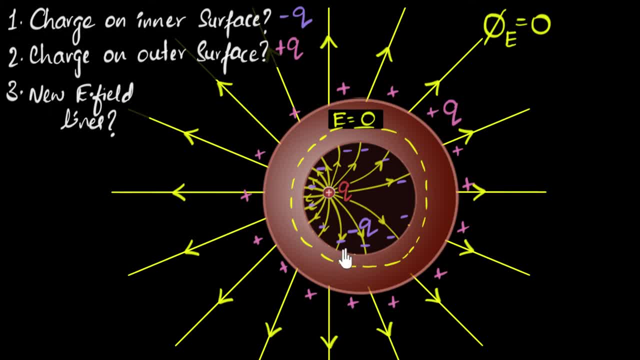 concentration, while some part is going to have less concentration again. can you pause the video and think about how the charge distribution would be on the inner surface? this negative q? all right, so because the charge is closer to this surface and you can see the electric field lines. 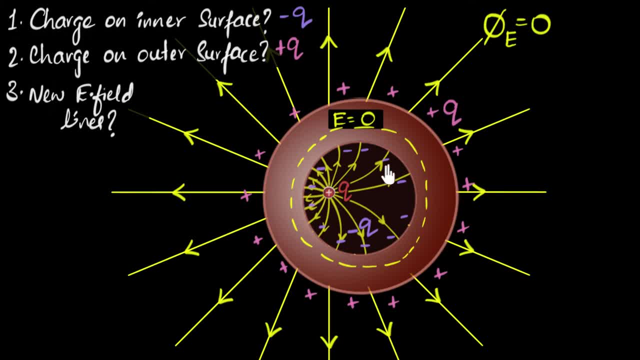 over here are stronger and they're close to each other and the electric field over here is far away and they're, which means it's weaker. we can immediately guess that the electric field lines are going to be more concentrated over here and there should be less, so you would have stronger. 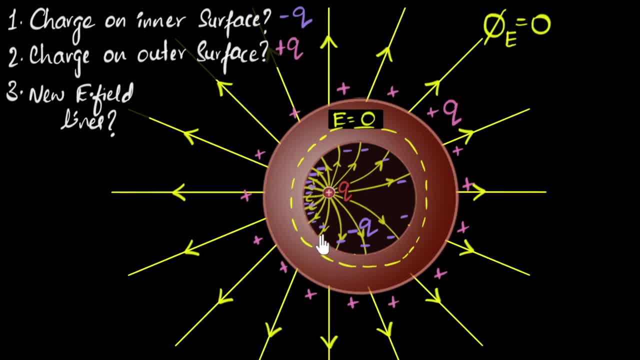 charge distribution. i know it's a little hard to see, but there should be more charges on this side and there will be less charges on this side, so charges will get more concentrated over here. so this will be less concentrated over here, all right. final question: how would the outer charge 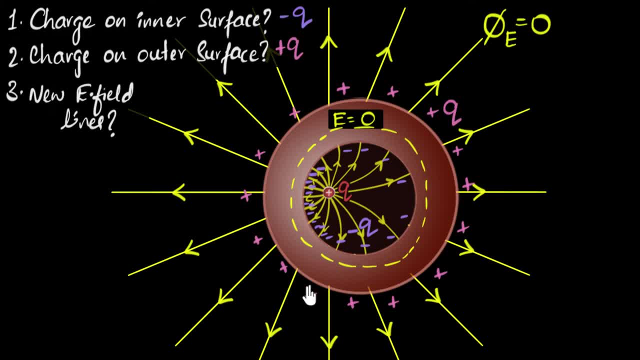 distribution look like. would it be uniform because it's a sphere, or do you think it's going to be? there'll be more positive charges over here, or will it be less concentrated over here, because there is more negative charge over here and there will be less positive charge over here? 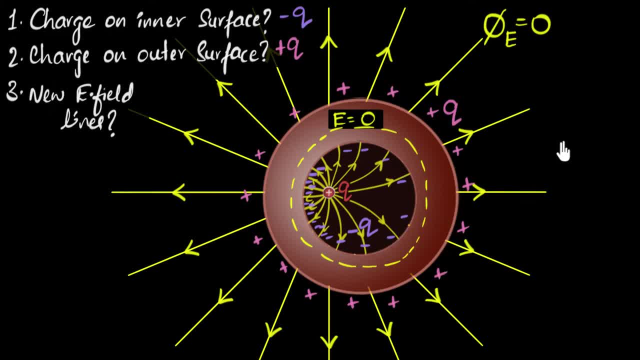 because there is less negative charge over here. so final time, can you pause and think a little bit about how would that be all right now? when i first thought about this, i thought, yeah, because there's a lot of negative on this side. there would be a lot of positive over here, a lot of positive.